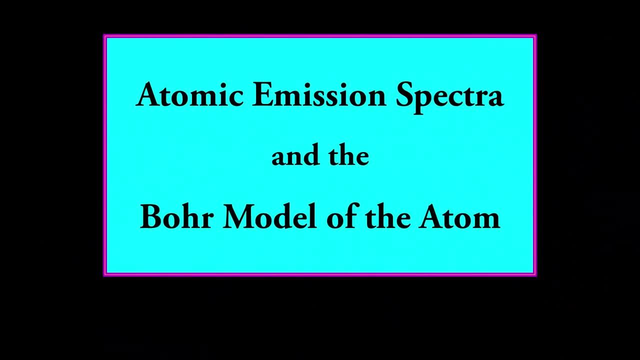 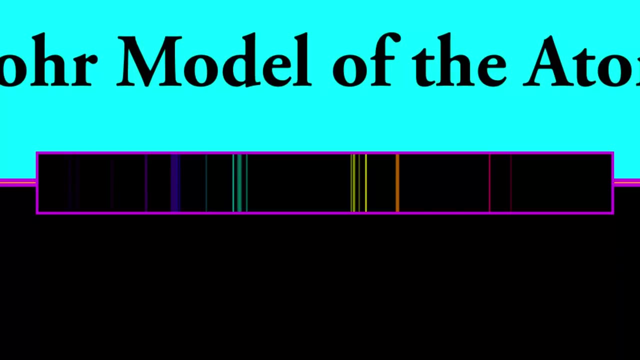 Welcome to Atomic Emission Spectra and the Bohr Model of the Atom. In the latter half of the 19th century, something remarkable was being noticed by a few scientists: Energized elements would emit specific visible colors of light, and the colors were specific to the element, but no one knew why this was happening. 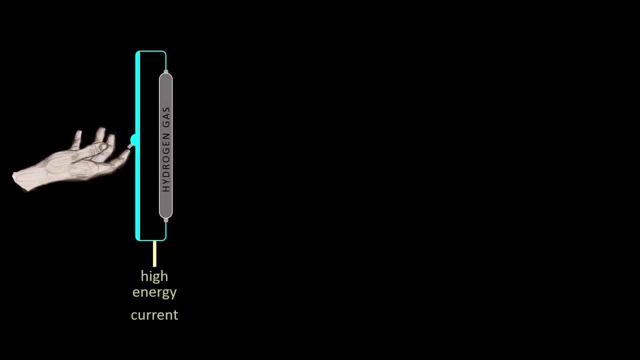 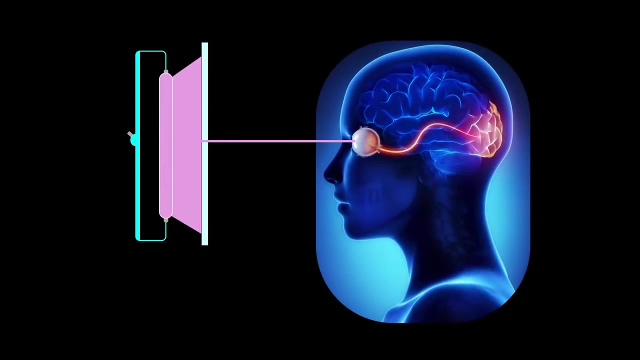 For example, if we energize hydrogen gas with an electric current, the hydrogen molecule is split into hydrogen atoms. Those energized hydrogen atoms emit a specific color spectrum of four colors. Our nervous system, however, is not able to see the four individual colors. 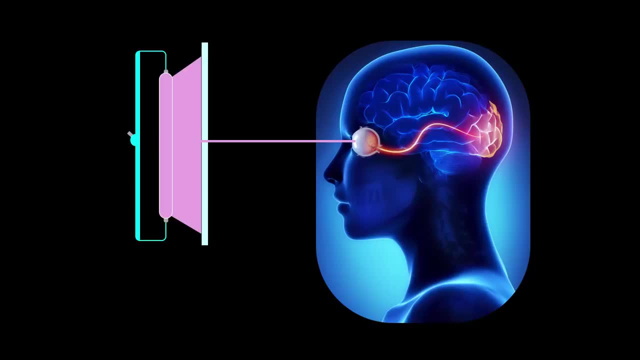 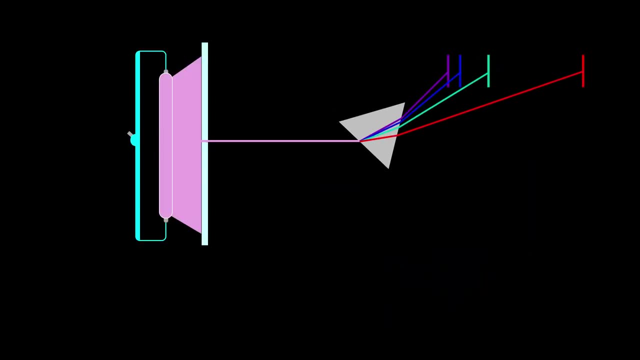 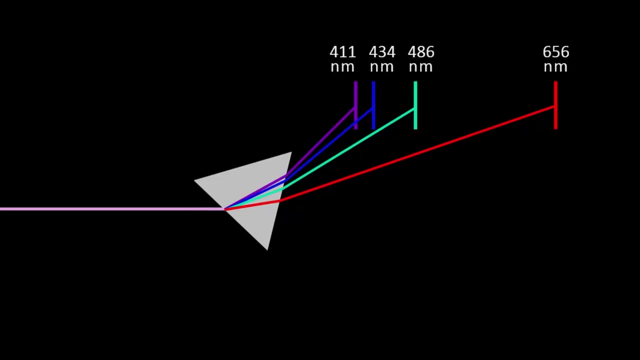 Our brain integrates those four colors into one specific color, and so that's the color we see. But when we diffract or split hydrogen's pale pinkish color, we can see the colors that are actually being emitted by hydrogen atoms: Violet, blue, a sort of turquoise and red all add specific wavelengths. 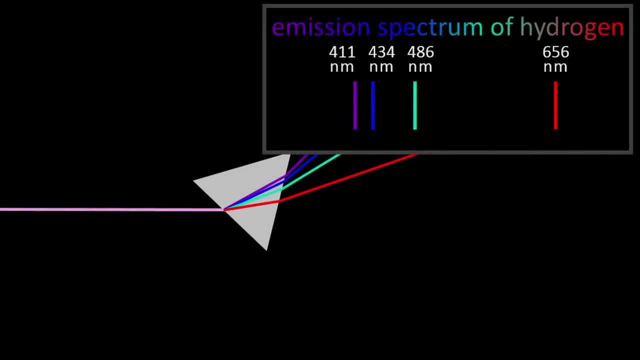 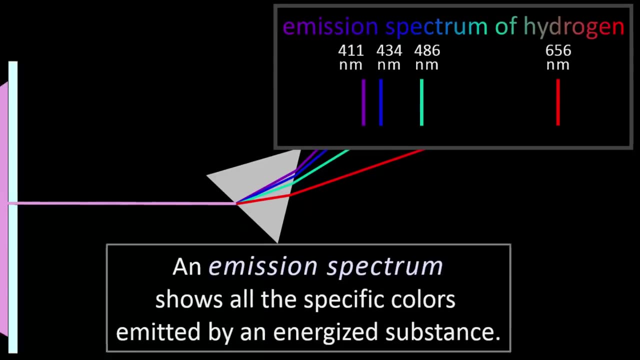 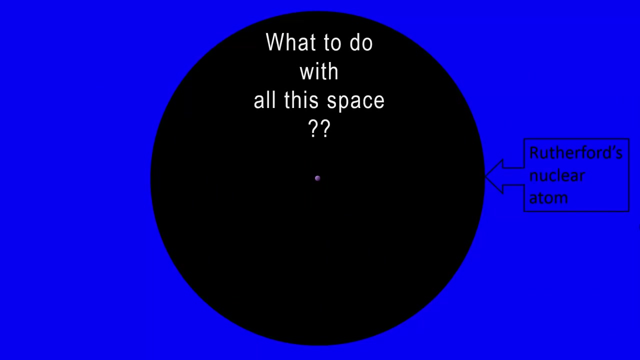 This is the emission spectrum of hydrogen. An emission spectrum is all the specific colors emitted by an energized substance. In 1913, using the atom's vast empty space provided by Rutherford's nuclear model of the atom, Niels Bohr used these spectral colors to create a model of the atom. 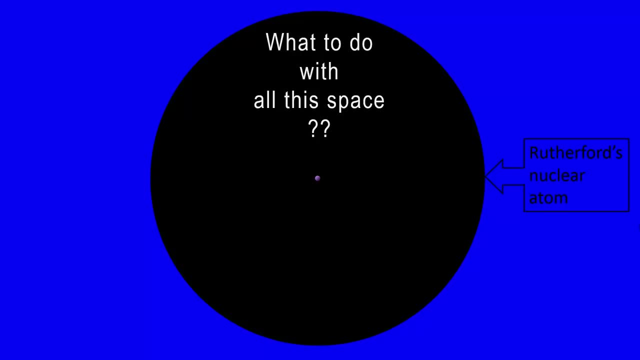 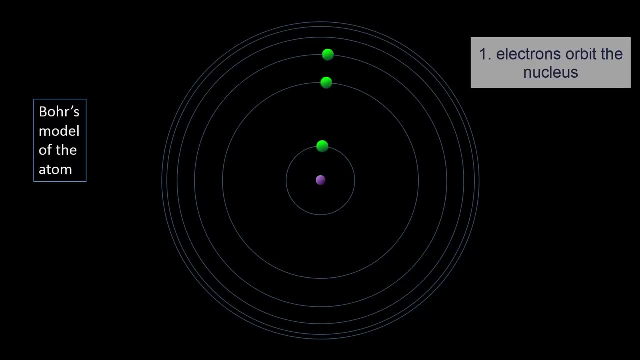 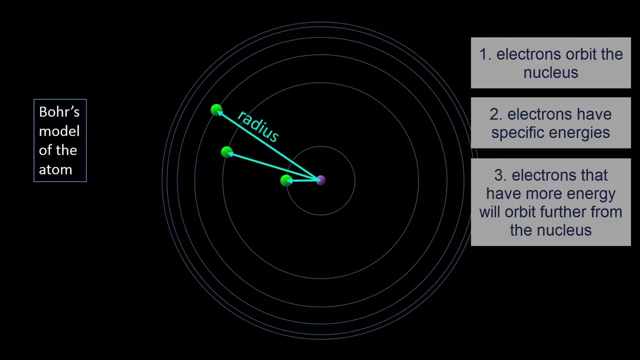 that explained the existence of the emitted colors and explained the behavior of electrons in the atom. In Bohr's atomic model, the electrons orbit the nucleus. The electrons have different energies and the higher their energy, the larger the radius of the orbit. 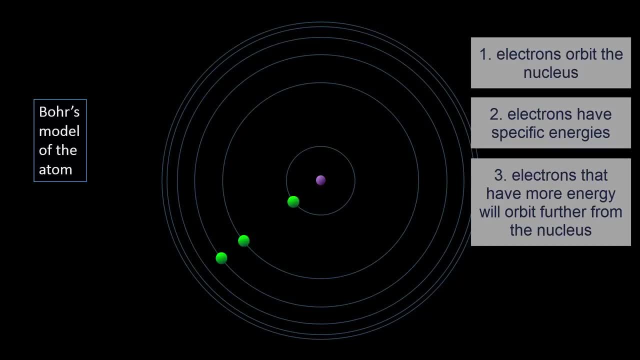 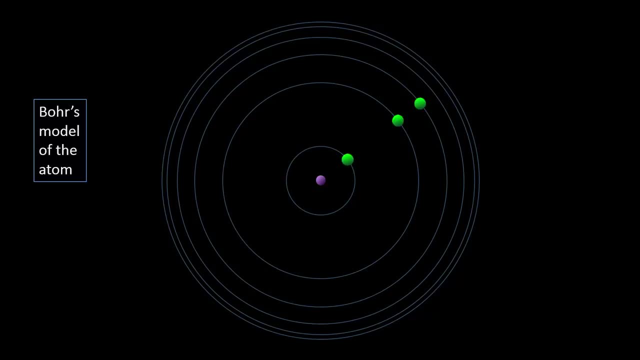 This model, however, presented a very large obstacle for early 20th century physics. It was known that an accelerating charge, which is what these orbiting electrons are, will emit energy in the form of light, and so that constant loss of energy would mean the electron would not be able to maintain an orbit. 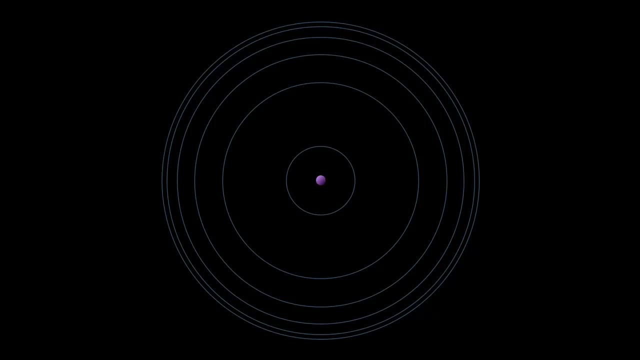 It would spiral down into the nucleus due to the strong attractive force of the nucleus. But Bohr said no, that would not happen. In his model, energy could be absorbed by an electron, putting it in a higher energy orbit, and the electron would only then emit energy. 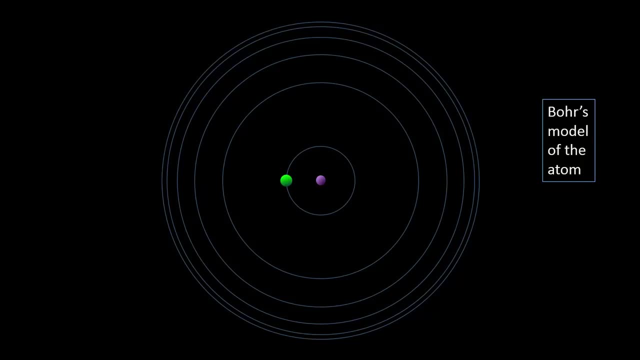 when the energized electron transitioned from a higher to lower energy. The energy of the emitted light is equal to the energy change of the electron. The emission spectrum of any one element is constant, and so Bohr concluded that the electrons can only exist at specific, discrete energies in order to produce such specific, discrete emission spectra. 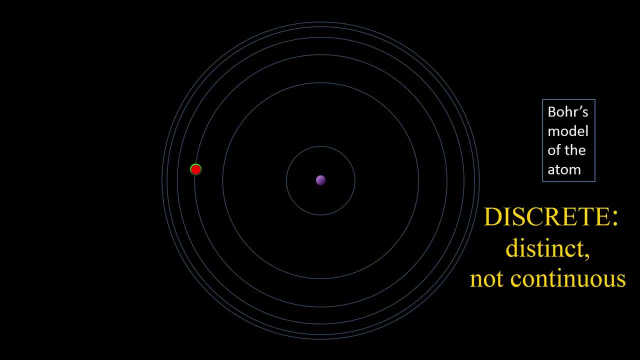 The electrons could not exist at energies in between these discrete energies, And this is what is meant by the term quantized electron. Let's take a closer look at this last idea, which was a contribution to atomic structure, which still holds true in our current quantum mechanical model of the atom. 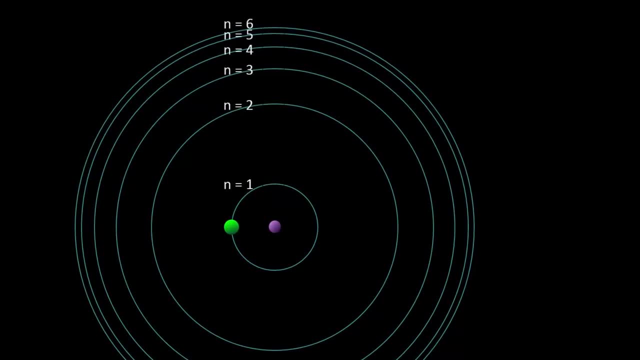 Bohr numbered his orbits with integers symbolizing each orbit, with the letter n representing the electron's energy. The letter n and the number came out of earlier mathematical analyses of alkali metals emission spectra by Johann Rydberg in 1888,. 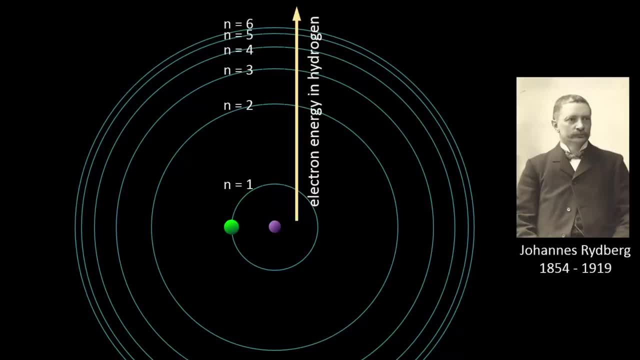 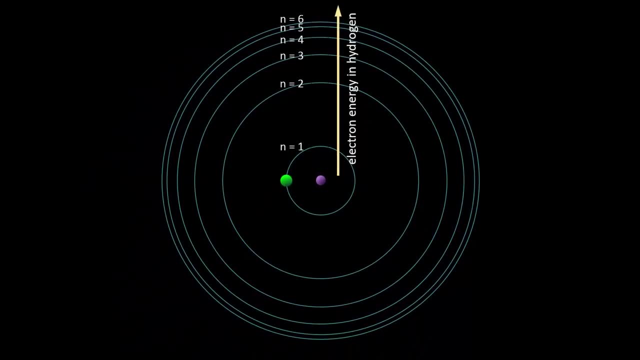 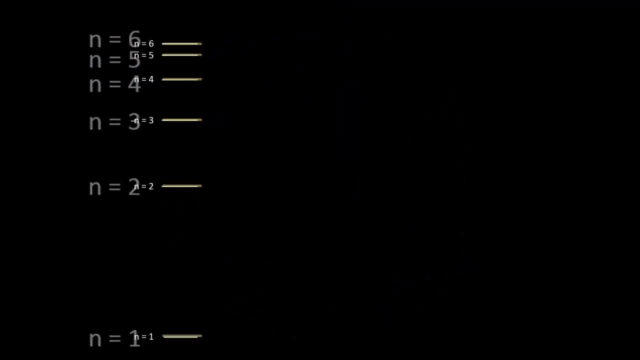 and so using integers is not arbitrary and they have mathematical significance which we will explore further a bit later on. If we focus on a section of the orbits, we get a diagram of the allowed electron energies in hydrogen Bohr found that these energies 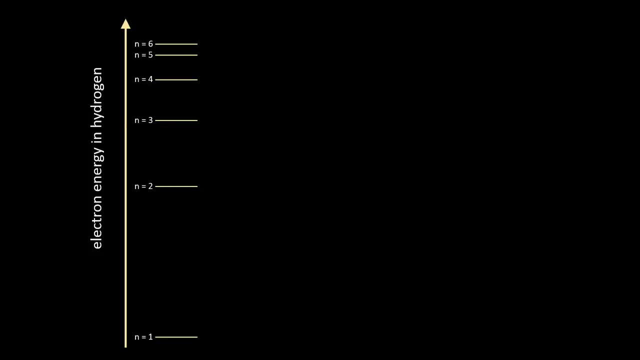 give us hydrogen's emission spectrum. An electron transitioning from n equals 3 to n equals 2, emits a red photon. From 4 to 2 gives a bluish green color, 5 to 2 gives blue and 6 to 2 gives violet. 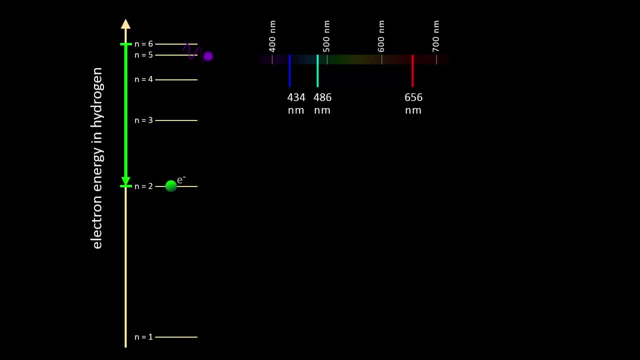 Notice that in the transition the electron does not exist in between those two allowed energies. If the electron could exist at any energy, then the change in energy here represented by delta E would result in emitting a large spectrum of colors, a continuous rainbow. 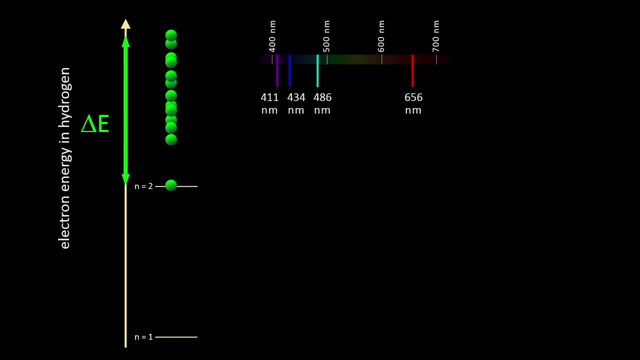 But only discrete colors are seen, and so the electron must remain at discrete energies. Again, this is called a quantized electron, an electron that can only exist at discrete energies. Bohr was very bold to tell the world that the electron was quantized. 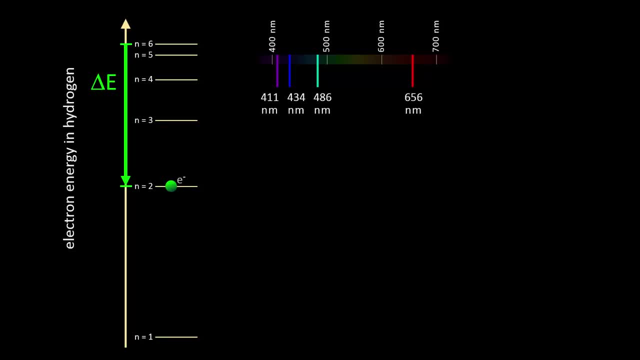 but there was the work of two other bold scientists to support him. In 1900, in order to solve a problem in the analysis of ultraviolet light, Max Planck came up with the idea of quantized light, energy being that light, in other words electromagnetic waves. 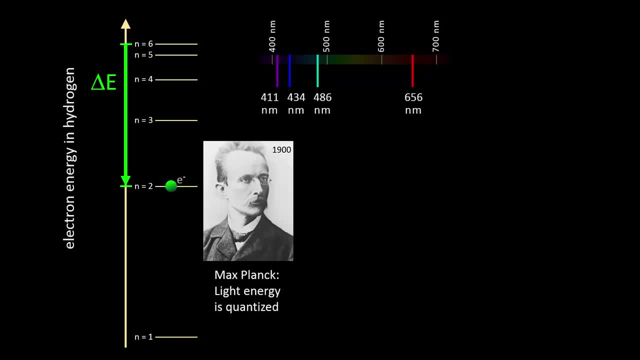 cannot have just any energy. they can only exist at discrete energies, which incidentally got him a Nobel Prize. Five years later, in 1905, Einstein took that a giant step further with his photoelectric effect, experimentally showing that light has momentum. 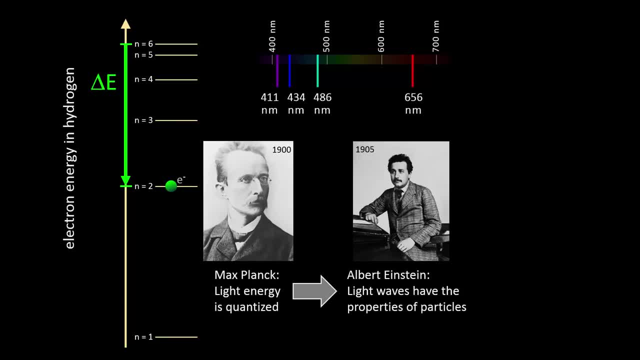 and momentum is a property derived from mass, but light has no mass. so the quantized light wave was behaving as if it was a particle, which we call a photon, which incidentally got Einstein Einstein a Nobel Prize. So, with the existence of quantized light behaving like a particle with mass, 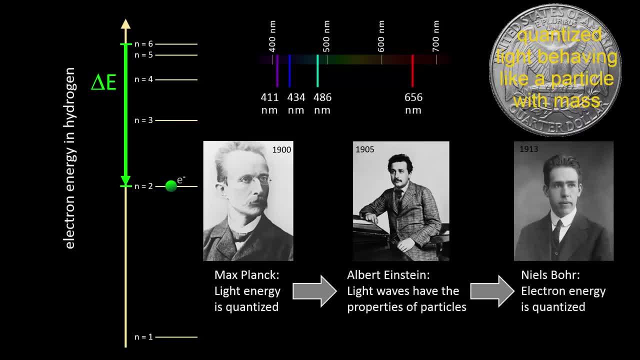 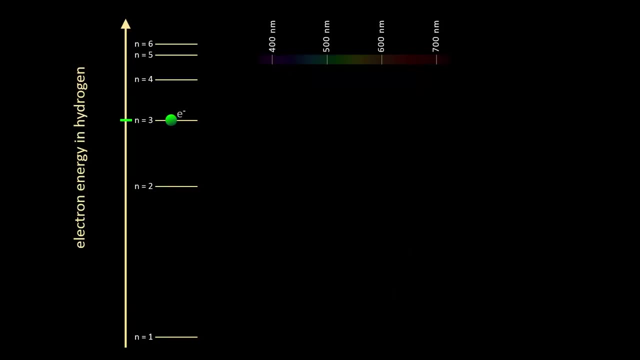 in 1913, Bohr looked at the other side of that coin and found that a particle with mass such as the electron could behave as if it was quantized. Yes, you guessed it: this got him a Nobel Prize. Let's take a more mathematical look. 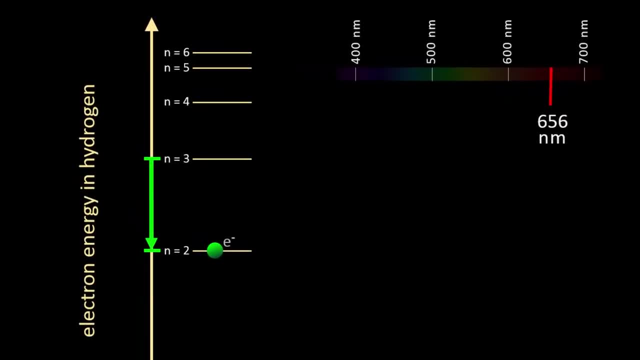 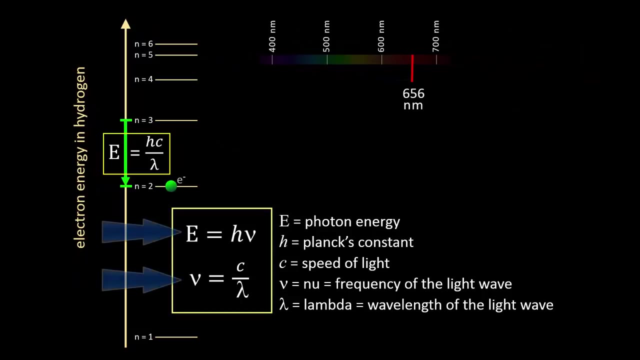 at the emission of red light from hydrogen. Let's mark the energy transition of an electron with an arrow and delta E. The energy of any electromagnetic wave can be calculated with hc divided by lambda, which is a combination of these two equations, by substituting c over lambda for nu. 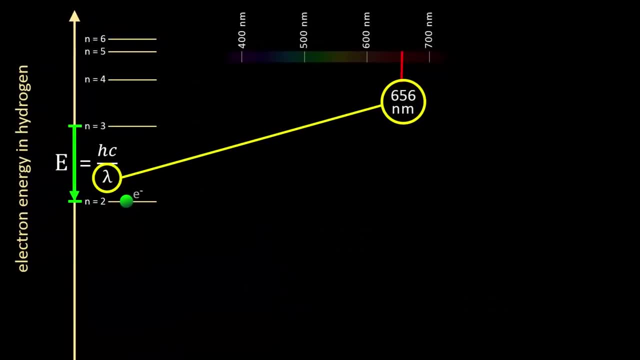 Given that we have the wavelength of the emitted red light and h and c are constants, we can then determine the energy of that red photon: Planck's constant h times the speed of light c divided by the wavelength, here expressed in meters. to keep units constant, 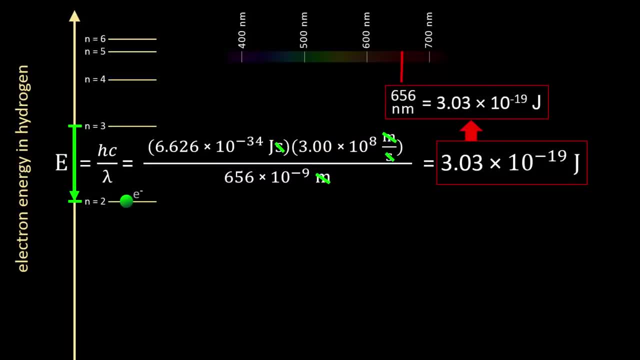 gives a photon energy of 3.03 times 10 to the negative 19 joules. In Bohr's model, that would also be the energy difference of the electron transitioning from n equals 3 energy to n equals 2 energy. The energy of an electron in hydrogen at any given n. 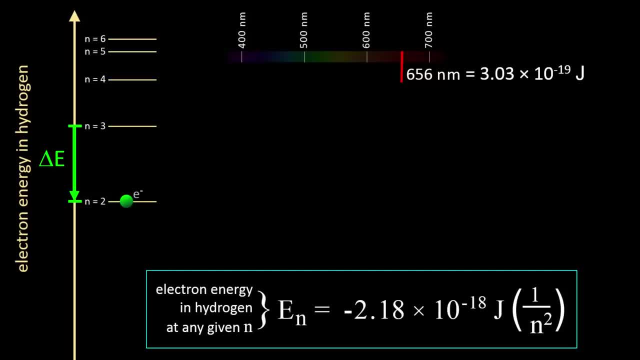 can be calculated using this equation derived from Rydberg's analysis of atomic emission spectra. Let's plug in the two integers from n to find the electron's energy at n equals 2 and n equals 3.. We may see something interesting For an electron at n equals 3,. 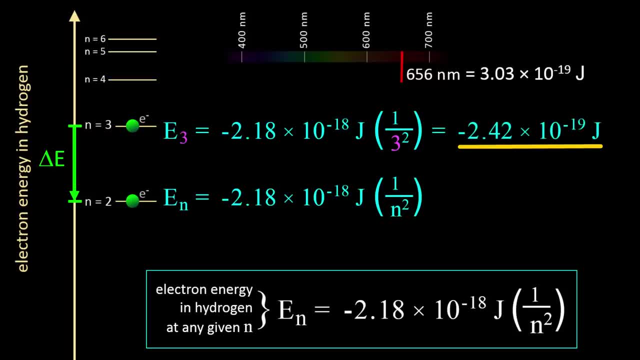 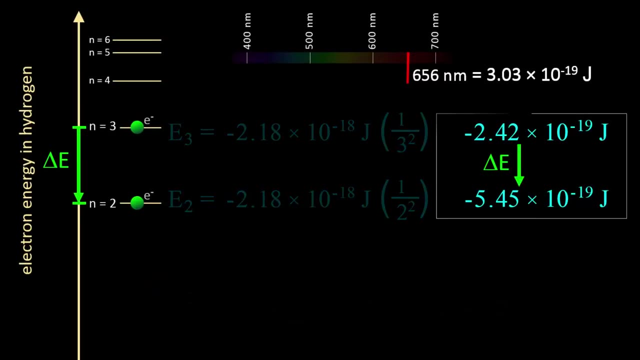 its energy is negative 2.42 times 10 to the negative 19 joules. For an electron at n equals 2,. its energy is negative 5.45 times 10 to the negative 19 joules. The difference between these two energies. 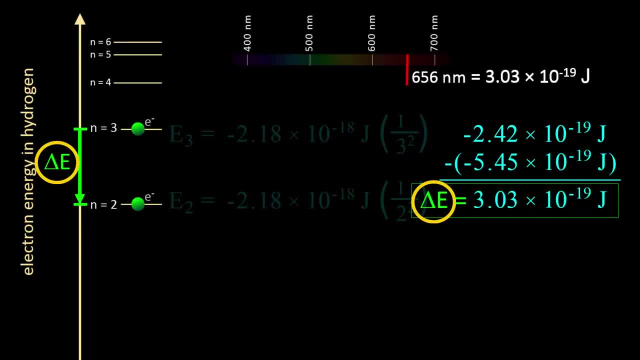 is the energy lost by the electron as it transitions from n equals 3 to n equals 2.. Which would be the energy of the emitted light. We can see mathematically that the energy lost by an energized electron when transitioning to a lower allowed energy level. 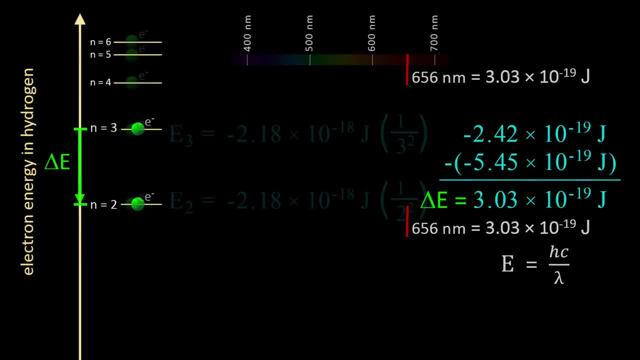 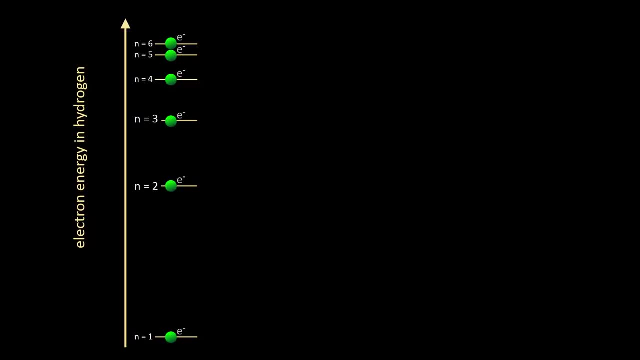 is emitted as light. So by determining the energies of emitted light, Bohr was able to work backwards and arrange the allowed energies of electrons by the magnitude of the transitions occurring to produce the observed emission spectrum. Note that the intervals between each succeeding n decreases as the electron energy gets higher. 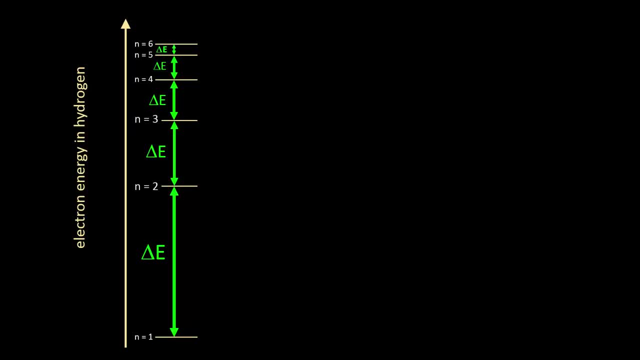 This came out of Bohr's analysis of light emission and is still an important part of our current quantum mechanical model of the atom, which begs the question: what else is there about the Bohr model that is still relevant to current understanding of the atom? 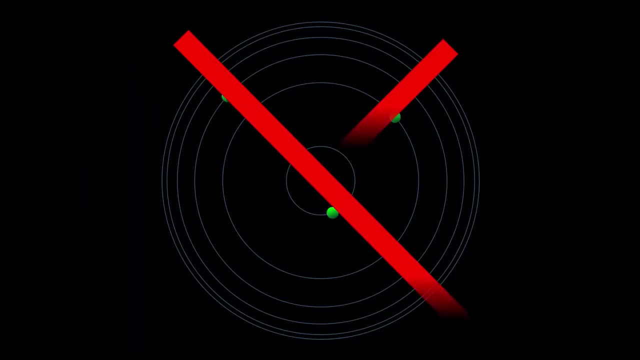 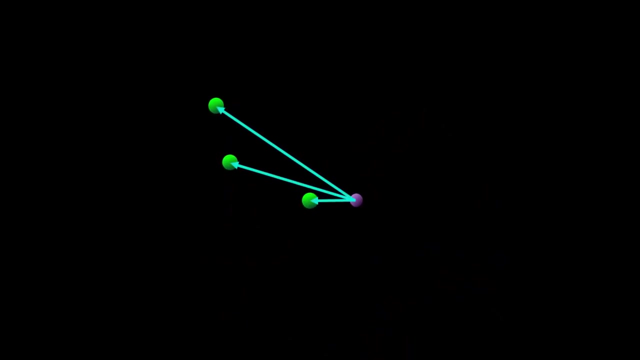 Well, we know that electrons do not orbit the nucleus, And that came out of Heisenberg's uncertainty principle 14 years later, in 1927, which, incidentally, was a part of Heisenberg's Nobel Prize. However, an electron's most probable distance from the nucleus